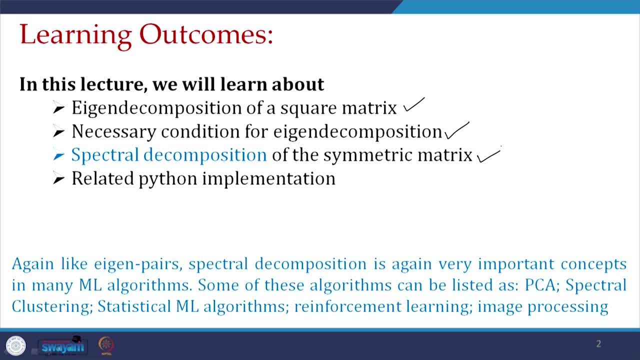 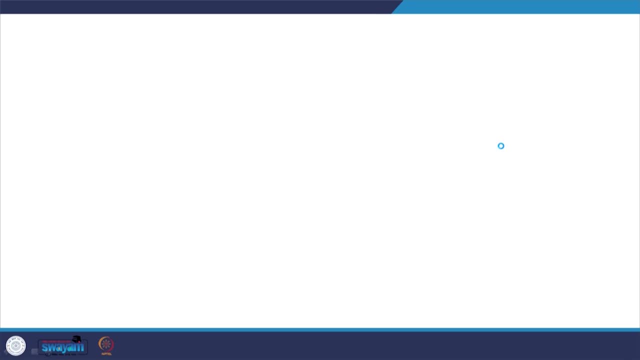 we make use of Eigen decomposition. It is also very important concept in case of when you are developing some recommender system. So, with this motivation, let me start with the definition of Eigen decomposition. 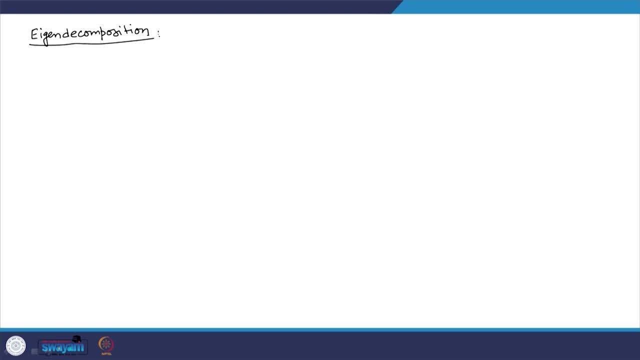 These are vectors and n-dimensional vector, space, and this is been the linearly. 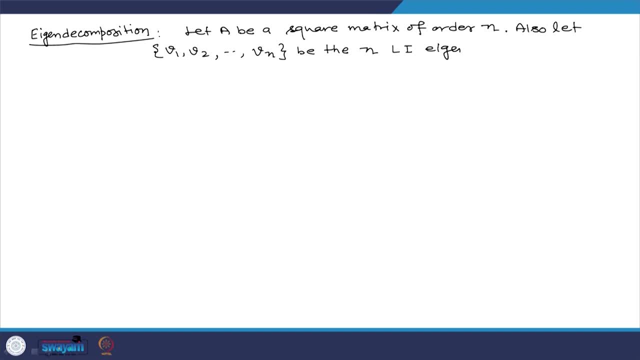 independent Eigen vectors of the matrix a, Then I can write these languages, only those drawing first. then other values are destroying each of them. A can be factorized as: A equals to n. invertible matrix P, a diagonal matrix D and the inverse. 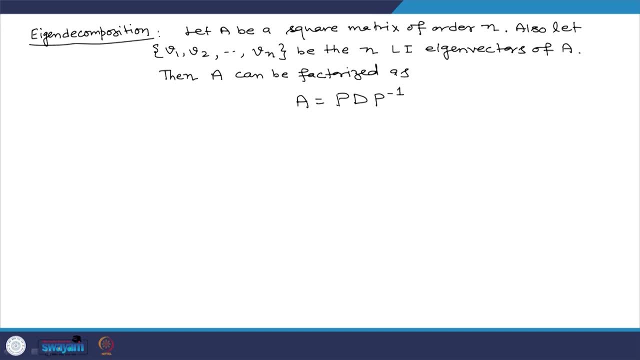 of P. So A equals to P, D, P, inverse. such kind of decomposition of A is called Eigen decomposition. Now what is the relevance of P and D with Eigen vectors and Eigen values of A? So the i th column of P is the Eigen vector V, i and it is an Eigen vector of A. So like how we are forming, 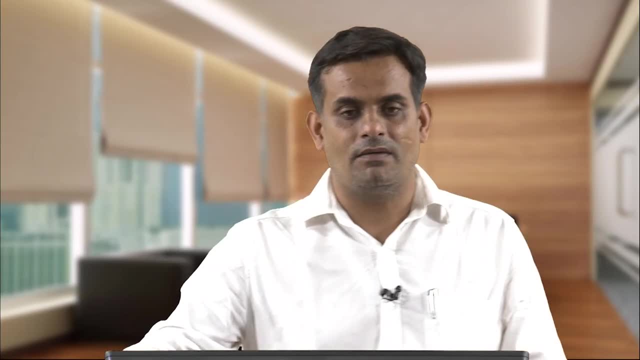 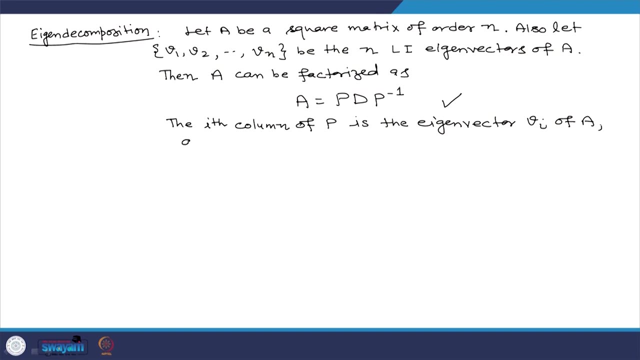 our matrix P, the first column is the first Eigen vector of A. second column of P is the second Eigen vector of A, and so on, And how we are forming D. So D is a diagonal matrix whose diagonal elements, which are 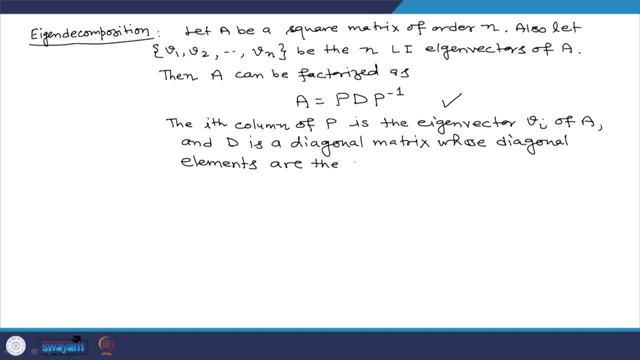 the corresponding Eigen value of A. It means D, i, i equals to lambda i If lambda 1, lambda 2 and lambda n, these are the Eigen values of A. So what is the relevance of P over omega z? Well, let us see how well we can estimate. 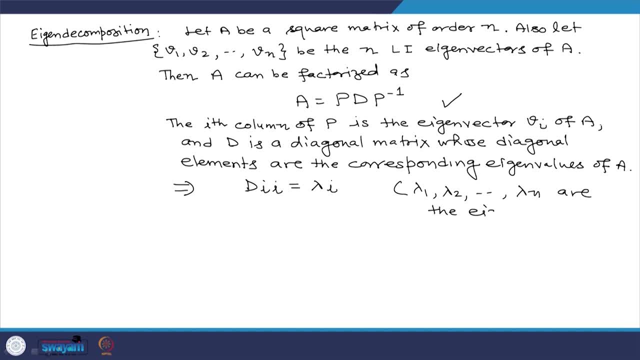 the relationship between A to P. In the previous lecture we had mentioned that B was the ranking vector of A. So in this particular example, let us say that A is the dimension of P and the venerable partner is B Here. the values of P: A is the denominator of P and 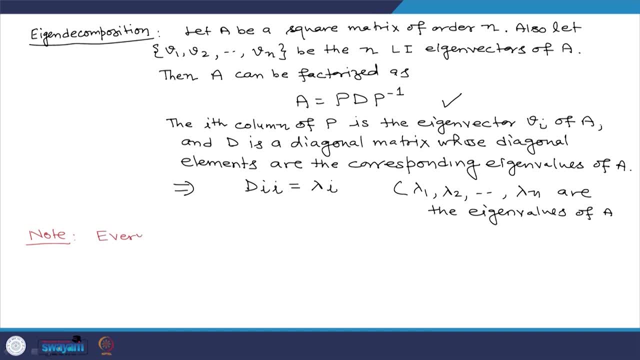 B is the vector of B. So the- this is what we are talking about for A, B of A. Now how So? every square matrix does not does not possess Eigen decomposition means you cannot make this kind of factorization like: A equals to P, D, P inverse, for every square matrix, A. 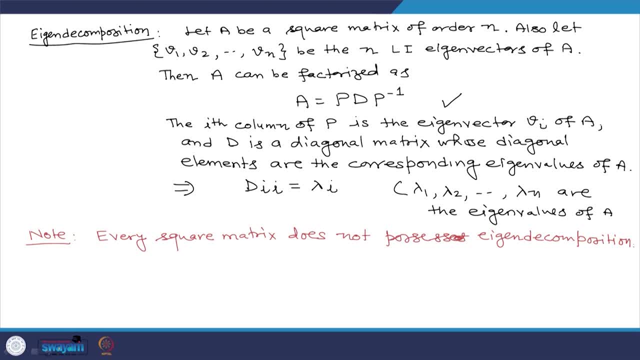 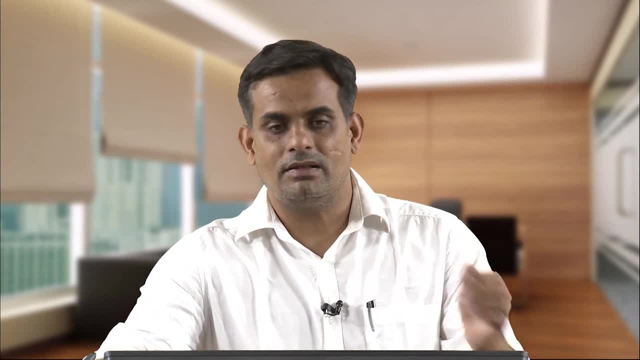 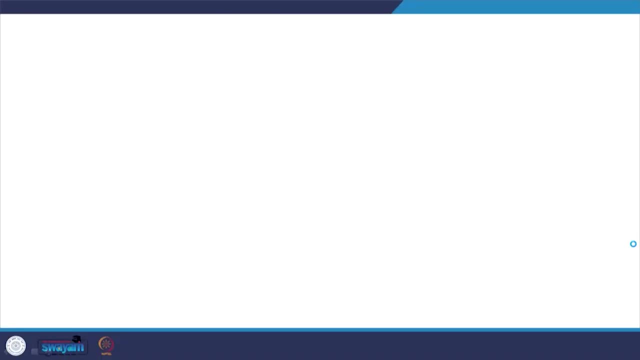 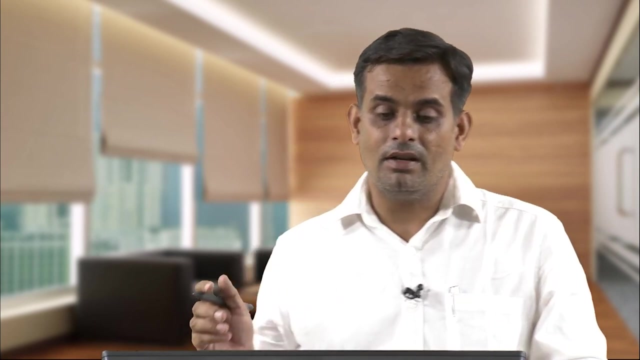 A matrix should have certain property, then only we can make this kind of decomposition. So what is that property? or in other words, what is the condition to have an Eigen decomposition? So before going to that The condition, let me give you an example of a 3 by 3 matrix for which we do not have Eigen. 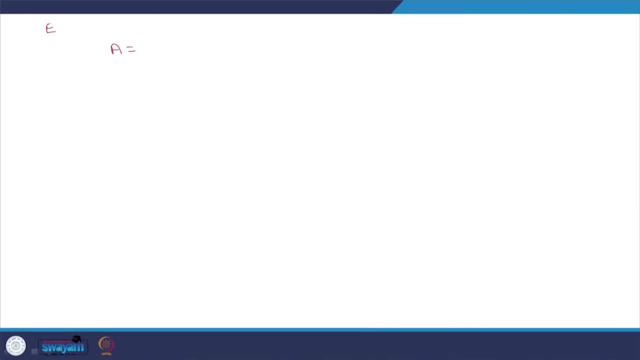 decomposition. So let me take A equals to 1 1 1 0, 1 1 0 0 1, so it is a 3 by 3 matrix And then, So it is a 3 by 3 matrix. 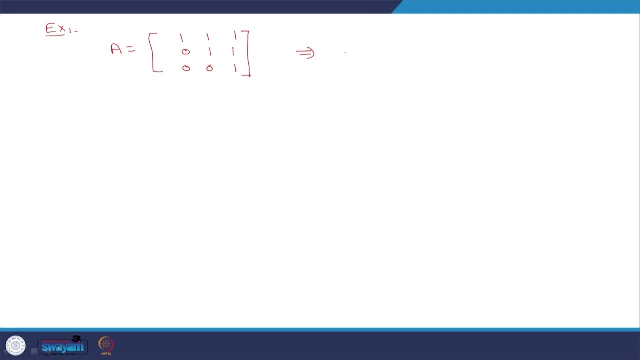 So it is a 3 by 3 matrix. Now, if you notice that it is an upper triangular matrix and in case of an upper triangular matrix the diagonal elements are the Eigen values. It means lambda equals to 1: 1. 1 are the Eigen values. 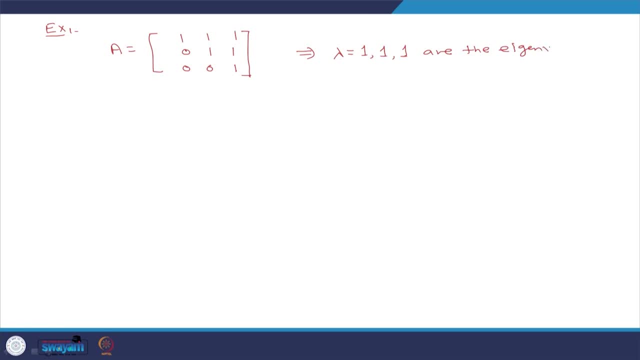 So that is a 3 by 3 matrix. So here you can see. So in other word, I can write that the Eigen value lambda equals to 1 is having algebraic multiplicity equals to 3.. As you can recall, the algebraic multiplicity is the number of. 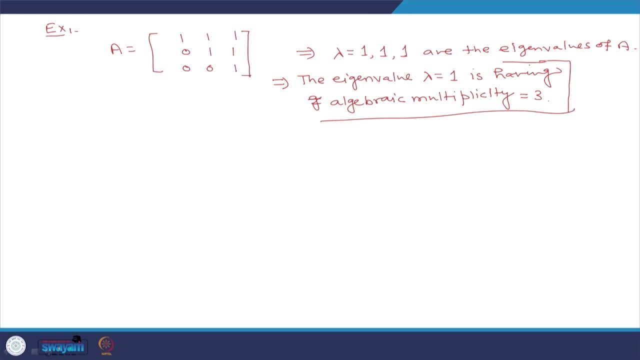 repetition of the Eigen value. Now let us check. the Eigen vector corresponding to lambda equals to 1.. So for calculating this Eigen vector, a minus lambda i times v equals to 0. Here lambda is 1.. So a minus i times v equals to 0.. Now let me write in matrix: 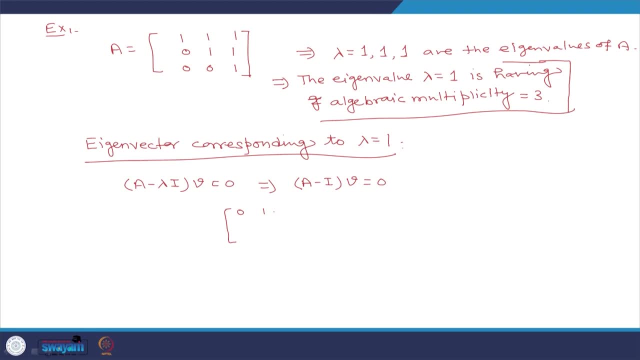 form a, a minus, i will become 0 1 1 0 0. 1 0 0 0 into v 1, v 2, v 3 equals to 0 0 0.. By solving this, you can have v 3 equals to 0. Then we will get the V 1, V 2, V 3.. We can calculate this: 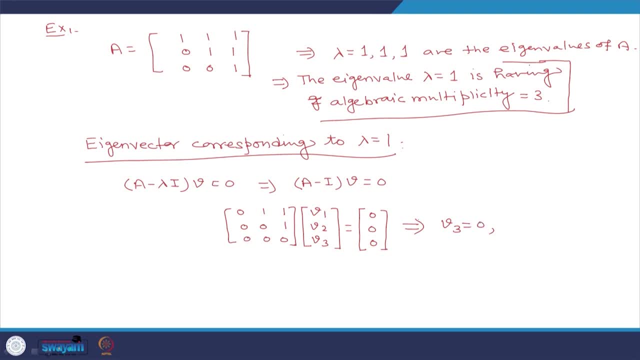 here We can see that the 29., 29. equation and then from the first equation, since V 3 is 0. So I am having V 2 equals to 0. So V 1 is arbitrary. So I can have only one linearly independent Eigen vector. 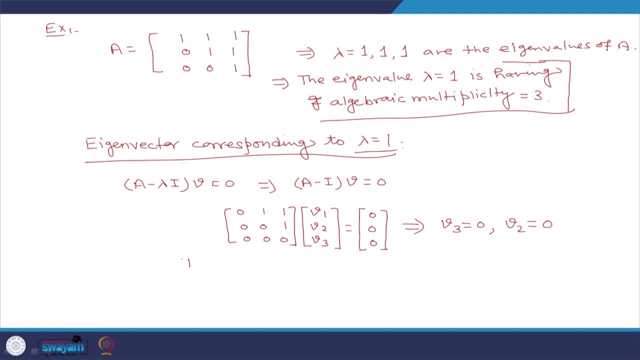 corresponding to lambda equals to 1.. So the geometric multiplicity of lambda equals to 1 is 1.. Now if I take V 1 as 1, the Eigen vector V is nothing, just 1, 0, 0.. In the previous 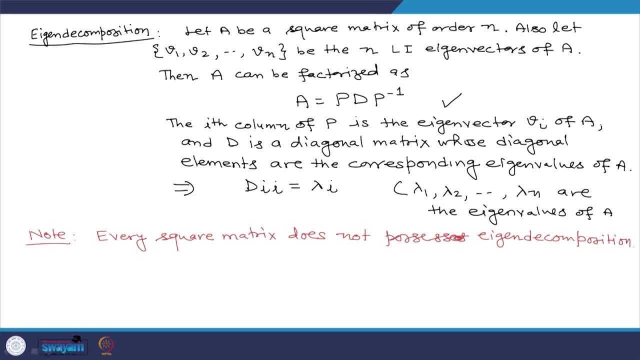 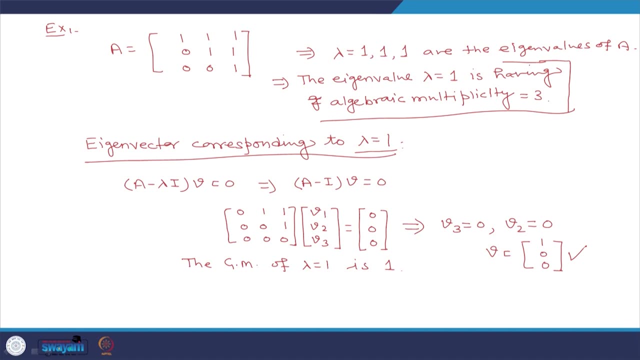 slide. I have told you that the columns of p are coming from the Eigen vectors of a. You are having only one Eigen vector of a, L i Eigen vector, So you can make only one column, but the size of p is 3 by 3.. So hence, 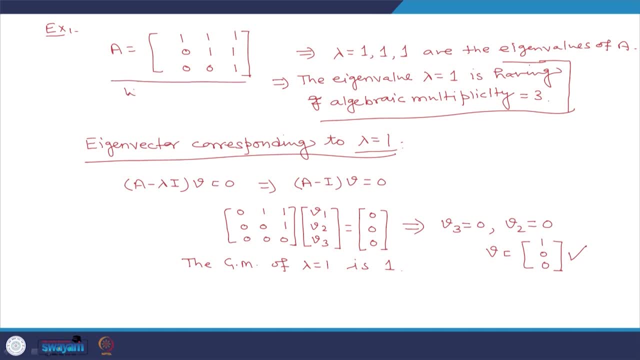 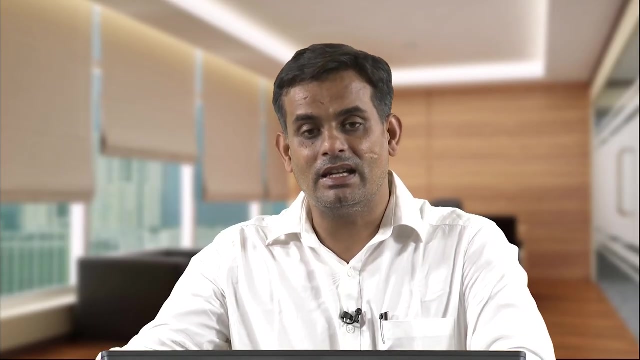 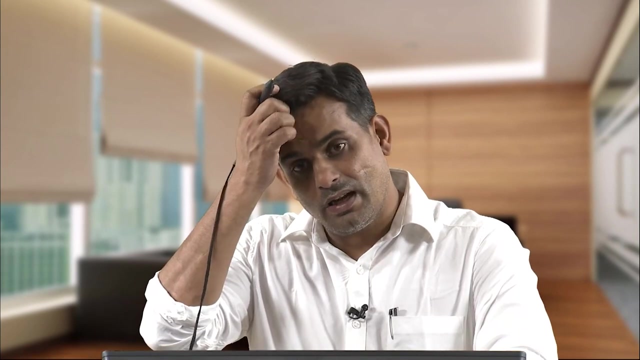 for this matrix. say we do not have Eigen decomposition. So what is necessary to have Eigen decomposition? if it is n by n matrix, then we should have n linearly independent Eigen vectors for that matrix. In case of each Eigen value, the algebraic multiplicity must be equals to geometric. 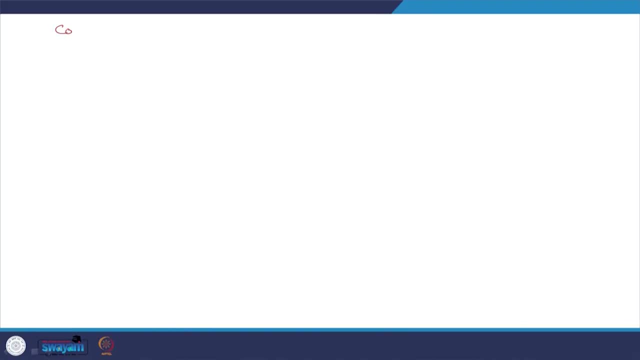 multiplicity. So now condition, let me write here. So what I can say: We need algebraic multiplicity to be equal to n. So what I can say is that we need algebraic multiplicity to be equal to n. So I am writing: n in short, equals to geometric multiplicity for each Eigen value. 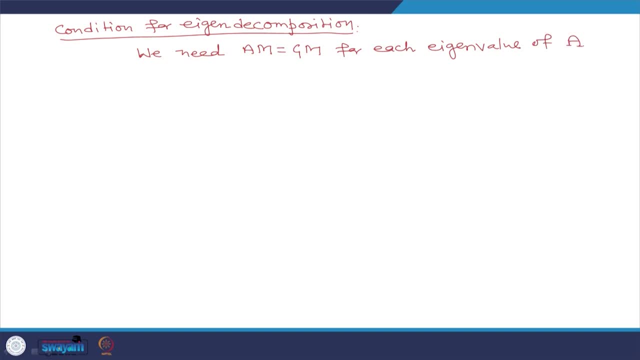 of a And if you sum all the algebraic multiplicity means in case of every Eigen value, then it will be equal to, Then it will be equal to n. So this is the algebraic multiplicity. then it will be equal to the size of the matrix. In other word, the matrix, say, should have 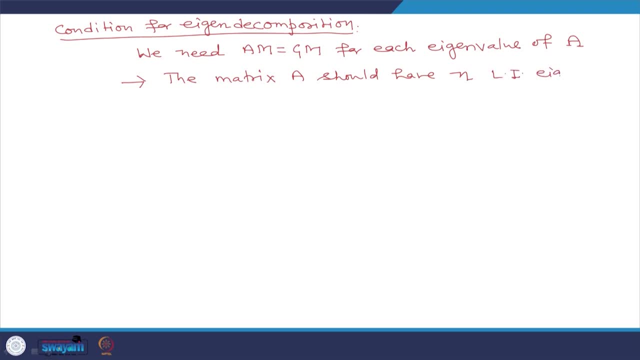 an linearly independent Eigen vectors, or in other word the Eigen vectors of A, forms a basis of a linear independent eigen vector And dimensional space. and dimensional vector- space on which the matrix A is defined- means it is a linear transformation. So this is the condition for Eigen decomposition. Now, 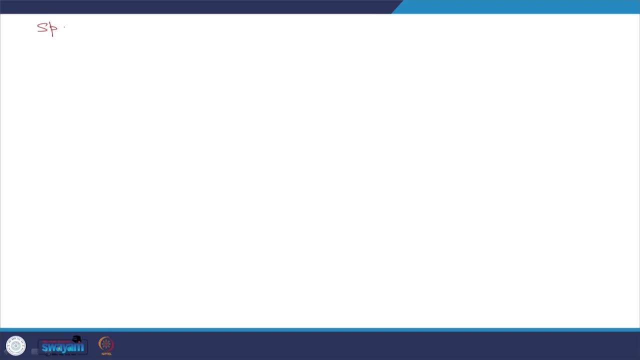 let me come to spectral decomposition, And this I am explaining. in case of symmetric matrices We are having more generalized class, like in case of Normal matrices, but here in machine learning, in most of the cases we use symmetric matrices. 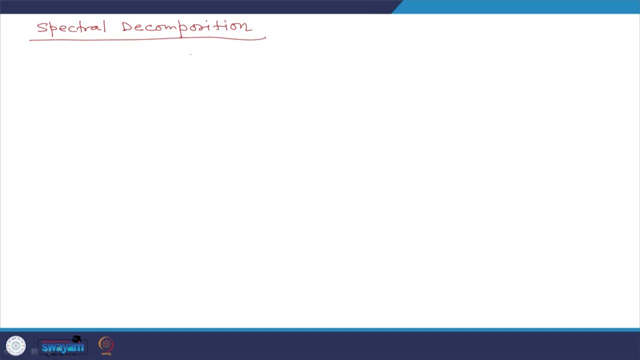 position in case of symmetric matrix. So let A, B, A, n by n- symmetric matrix- then the Eigen decomposition of A is guaranteed. Why I am saying: for every symmetric matrix, you can perform the Eigen decomposition for every symmetric matrix. 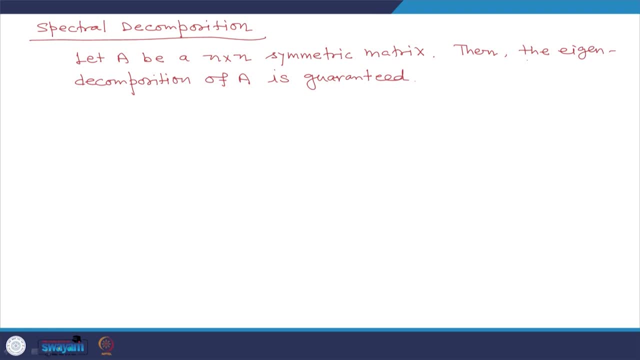 You can perform the Eigen decomposition Now. this means I can write A equals to P, D, P inverse. Now consider lambda 1, lambda 2, lambda n are the. Now, by this Eigen decomposition I can write A equals to. I will write P, P is nothing. 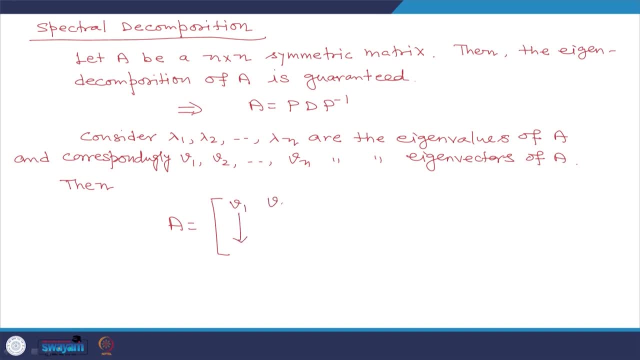 You take first Eigen vector is the first column of P, V, 2 and so on up to n, into the diagonal matrix D, where diagonal entries are Eigen values of A. rest of the entries are A. So this is the diagonal matrix. The rest of the entries are 0, and then P inverse. So this is your P inverse of this. Now the 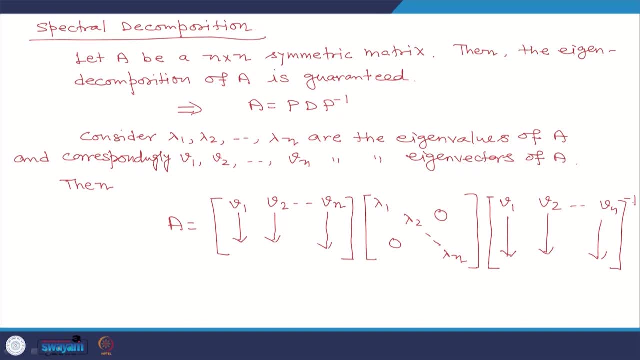 Eigen vectors of a symmetric matrix. it is not only a lie, but orthogonal. You will be having orthogonal Eigen vectors for a symmetric matrix matrix. It means v 1, v 2, v n forms an orthogonal set of Eigen vectors means v 1, dot. v 2 is. 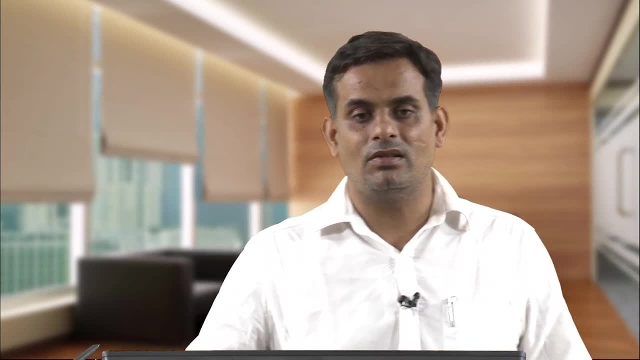 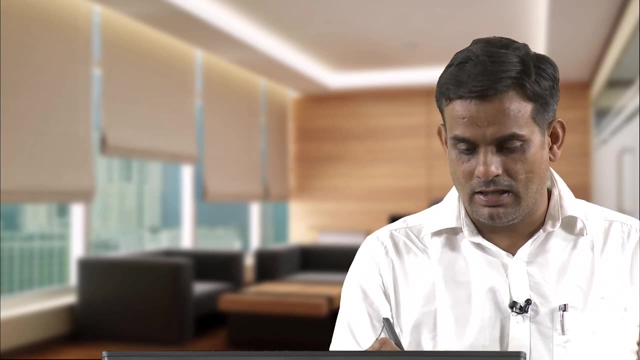 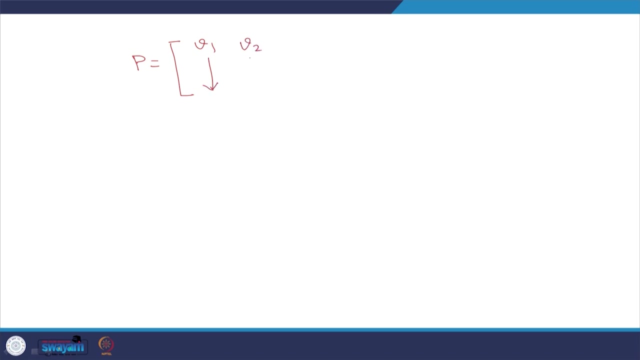 0, v 1 dot, v 3 is 0 or, in general, v i, dot, v, j is 0 when i not equals to j. So in that case the matrix P, which is having these orthogonal vectors as the column, is an orthogonal matrix. 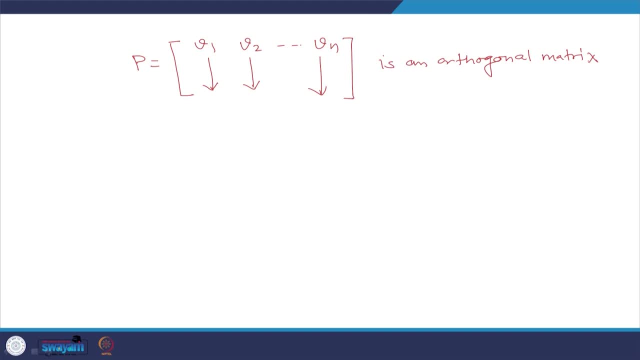 Means every square matrix which is having orthogonal columns is orthogonal. It means that P inverse equals to P transpose. It means the Eigen decomposition of A can be written as P d, P transpose. Now I can write it: A equals to v 1, v 2, v. 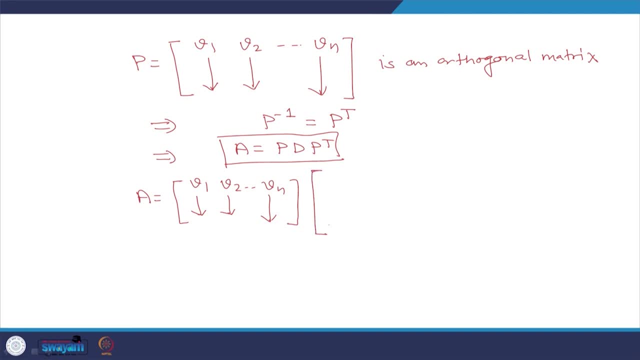 n, Then lambda 1, 0, 0, 0, 0, lambda 2, 0. this matrix b and then P, transpose each First column will become first row v 2, v n. So if I multiply it, I can write: A equals to: 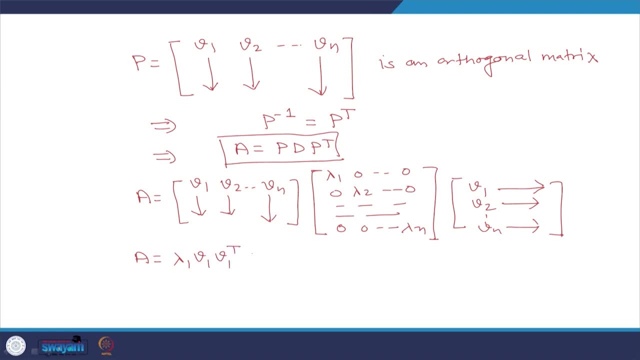 lambda 1, v 1, v 1, 2.. And if I include a number of 1s is equal to lambda 2, it would tell lambda 2.. This is transpose plus lambda 2. V 2, V 2 transpose plus lambda n. V n, V n. transpose where if 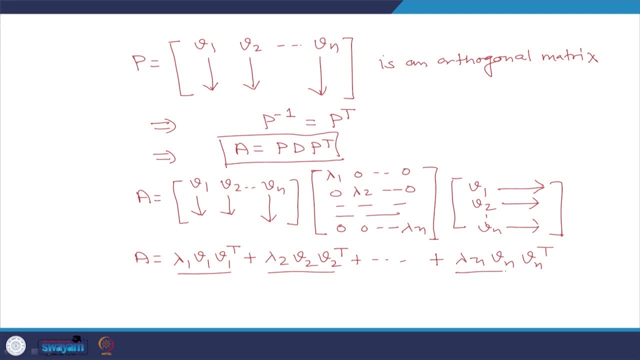 you see each term of this summation. what is this? It is a matrix of rank 1, rank 1: n by n matrix. Similarly, again, it is lambda: 2 V, 2 V, 2. transpose is again rank 1: n by n matrix. 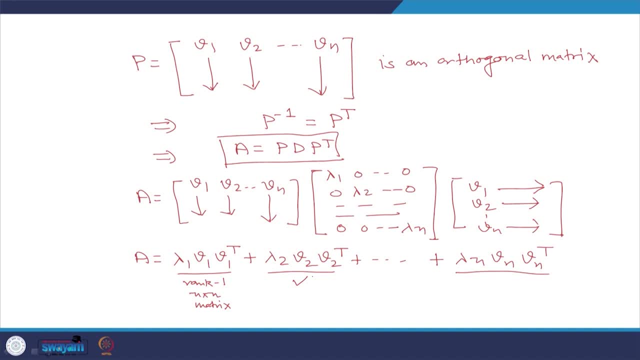 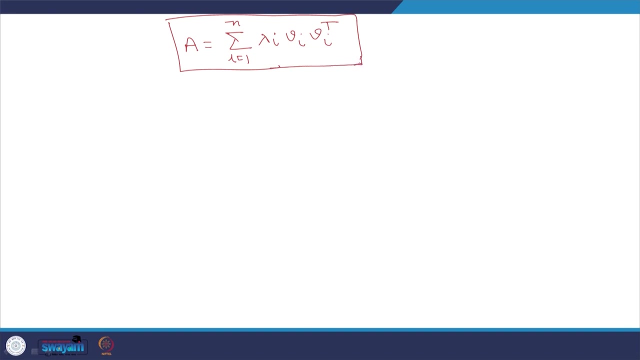 and so on. So each of these term is rank 1, n by n matrix. So I am having a equals to summation, i equals to 1 to n, lambda, i, V, i, V. i transpose So such kind of decomposition of A into a sum of n rank 1 matrices is called spectral. 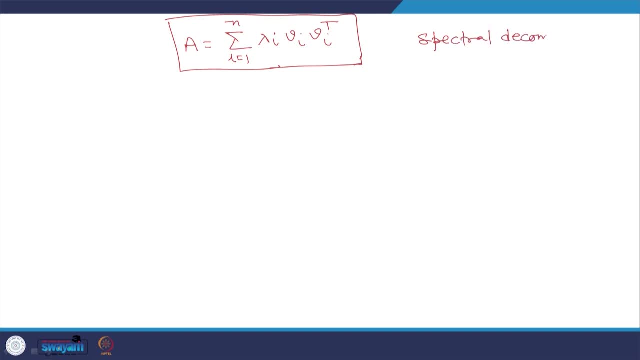 decomposition of A. Now an special note or remark. Each matrix V i, V i transpose for all i equals to 1 to n is the projection on to one dimensional sub space. Sub space of parent is spanned by which one V i. So means we are having: 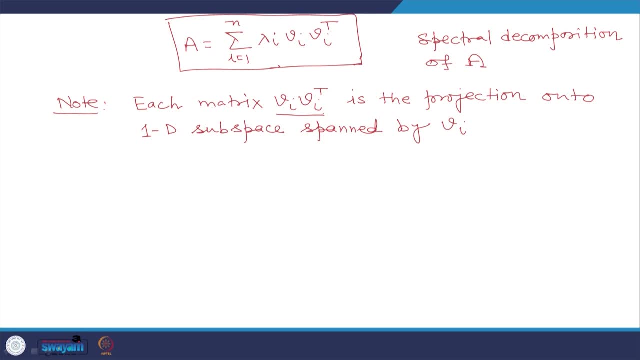 each of this matrix is a projection transformation on to a sub space which is spanned by V, i In other where I can write, if I am writing this projection matrix, A, P. So this linear map P operating on X equals to V i, V j transpose X. So this V i V j transpose, which is equal. 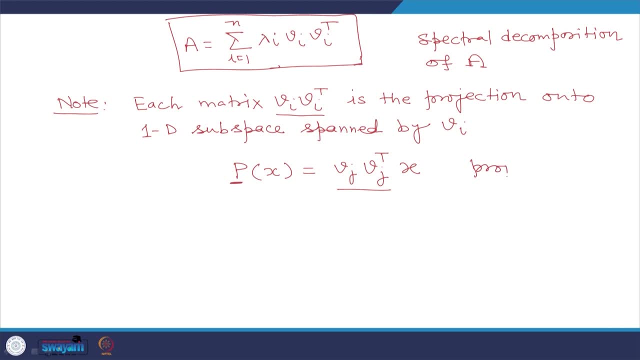 to P is a projection map, And what kind of it is. So it is an orthogonal project. So it is a projection on to the sub space, expand by the Eigen vector v, j. So let me close this. 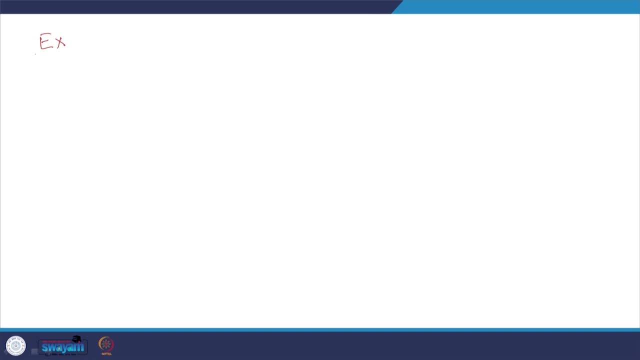 lecture with an example. So a very quick example let me take. So consider a 2 by 2, matrix A which I am taking: 2 1, 1, 2.. So I will show you the Eigen spectral decomposition of A, The Eigen value. you can. 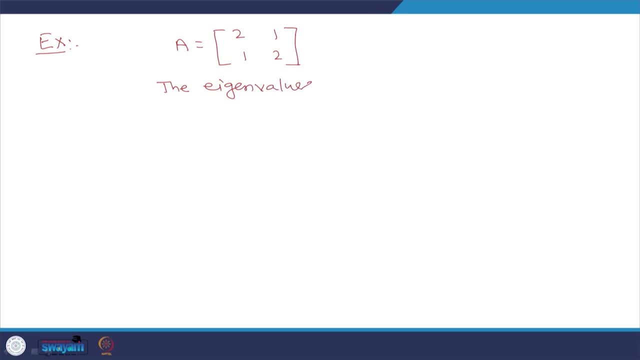 calculate. you are familiar with Eigen value. So Eigen values of A are 3 and 1.. So let us say 3 is lambda 1, 1 is lambda 2.. of A are means corresponding to lambda 1: 1, that is 3 is v, 1 equals to 1, 1 and v 2 equals. 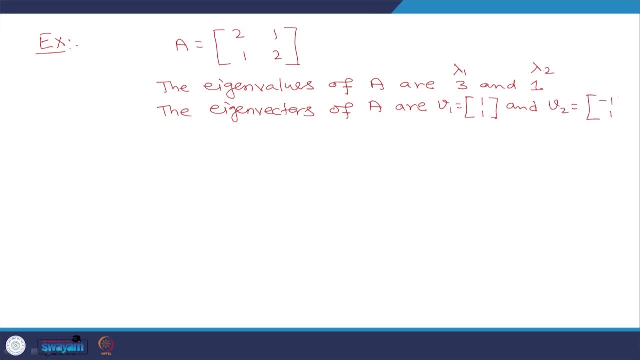 to minus 1, 1.. Now what you do? You can verify this: v 1, v 2, v 1 dot is equal to 3.. So you v 2 equals to 0, means they are orthogonal vectors and it is obvious because they are. 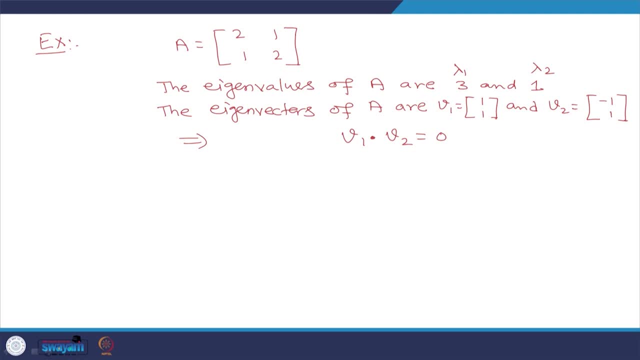 Eigen vectors of asymmetric matrix. Now let us make them orthogonal. So let me write: v 1 equals to 1 by root 2, 1 by root 2.. So each element of v 1 I have divided by the length of v 1 and v 2 equals to minus 1 by root 2 and 1 by root 2.. It means I can. 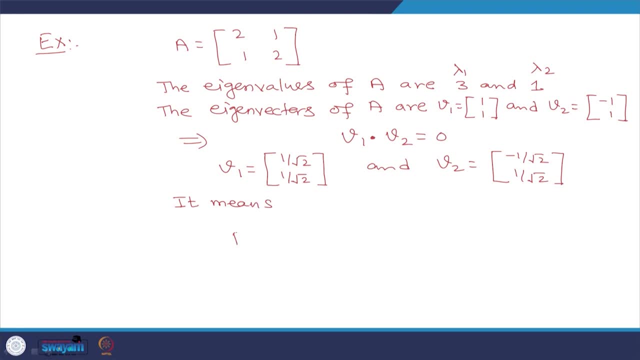 write my p and d, So p equals to you. write v 1 as a column, So 1 by root 2, 1 by root 2 minus 1 by root 2, 1 by root 2.. Then you can have d equals to lambda 1, 3, lambda 2: 1, 0, 0.. Then is this Eigen decomposition. 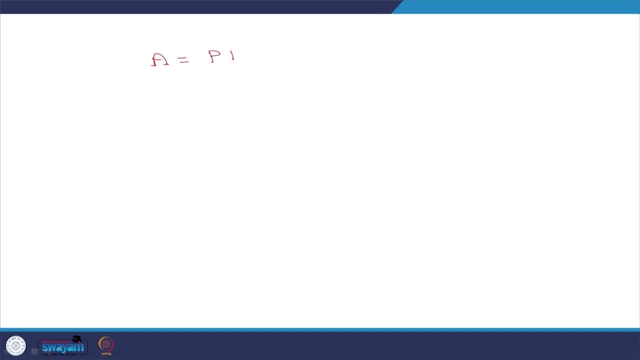 irrespective decomposition of a p, d, P. transpose it means it is 1 by root 2, 1 by root 2, minus 1 by root 2, 1 by root 2 and 1 by root 2.. So if we write all these, we will end up with the following of решил decentralization. 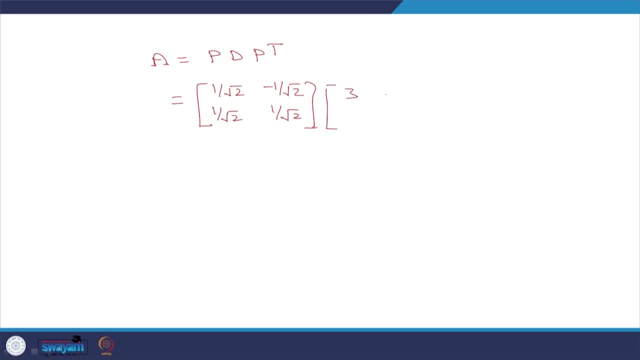 and then, as you are left with the essential combination in A, D, E and K plus m into 1 by root 2, 3, 0, 0, 1 into naught: 1 by root 2, the transpose of p. Now the spectral decomposition. 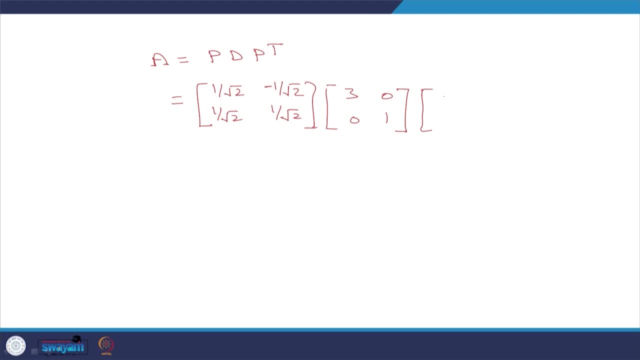 of a can be written as lambda 1, V 1, V 1 transpose, plus lambda 2, V 2, V 1 transpose. So this is V 2 transpose. So V 1 into V 1 transpose will be, So let me do it here. So V 1 is. 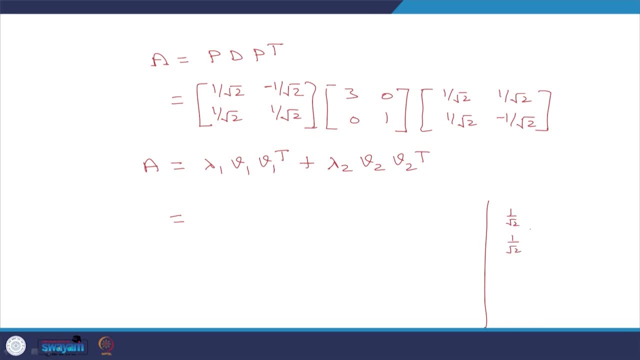 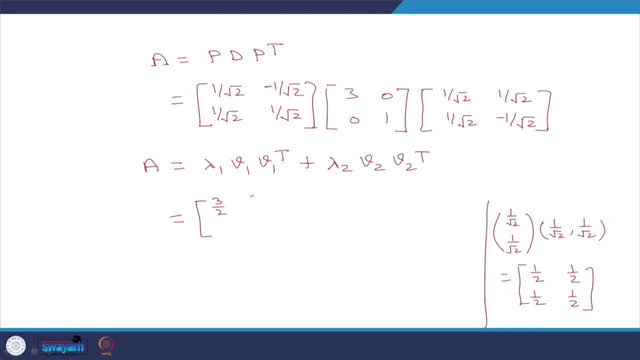 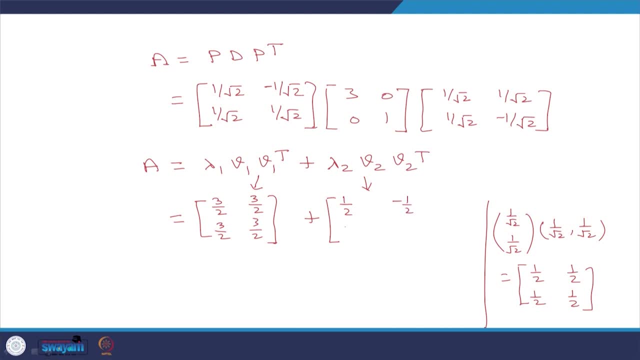 2 minus 1 by 2. This is again minus 1 by 2, and 1 by 2 means similarly, you can write, you can calculate it. So now you can see this: 2 are nothing, just projection matrix, And it is the spectral. 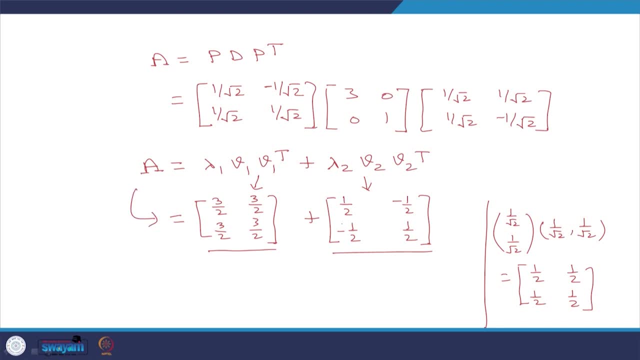 decomposition of a. You can add this: 2. You will get the matrix A. It is also having rank. 1. You can easily see both rows or both columns are same. They are l d and here also both the columns are l d. 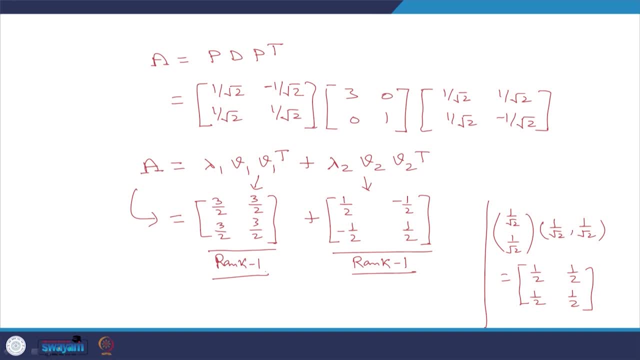 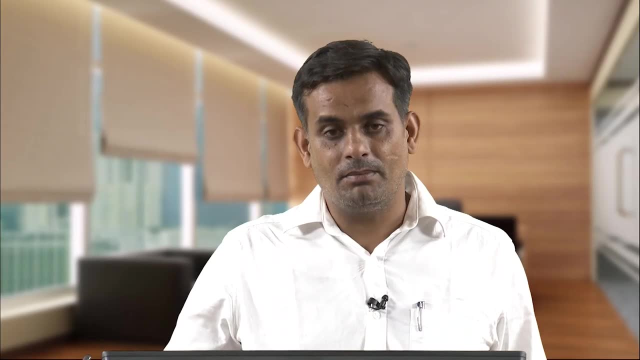 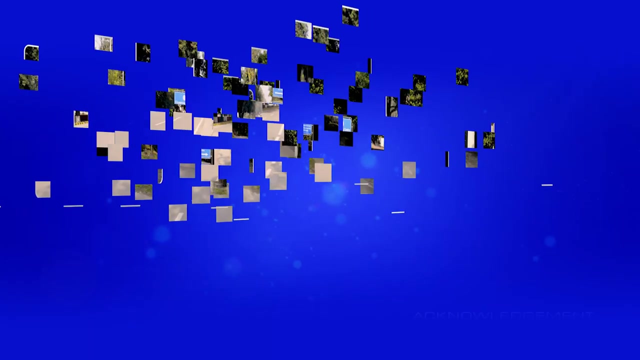 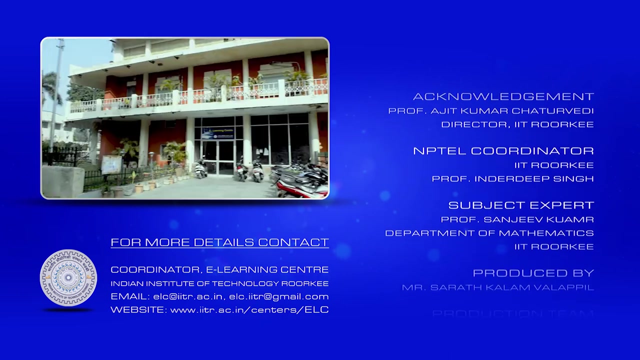 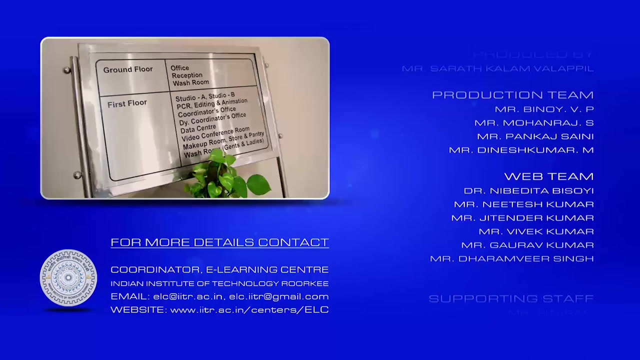 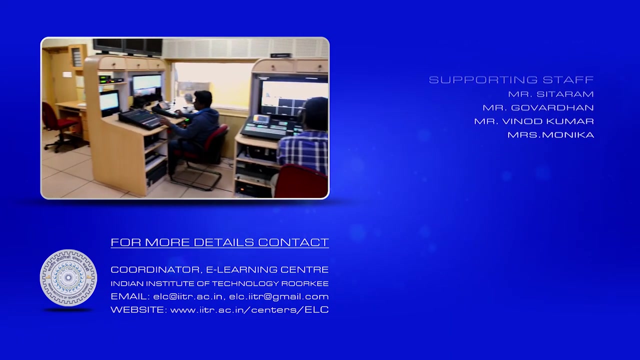 the, so rank 1.. So this: in this way we can calculate the spectral decomposition of A. so with this example let me close this lecture. Thank you very much, Thank you.